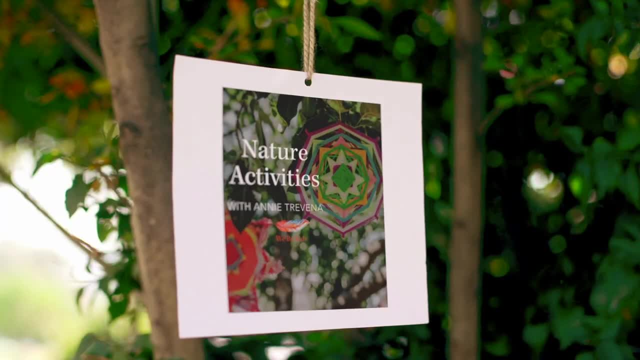 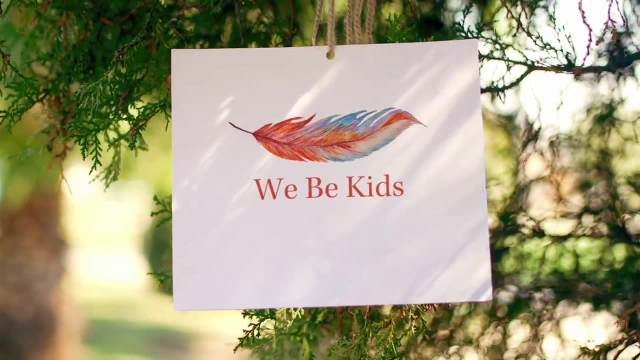 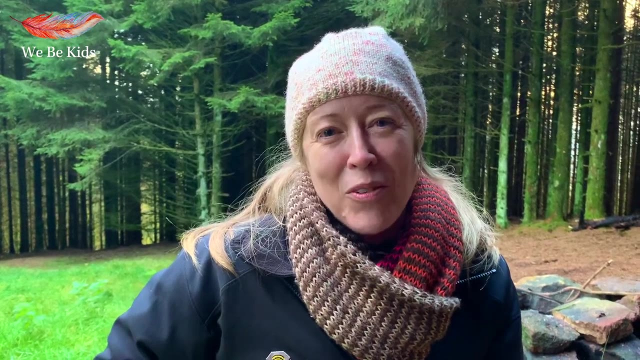 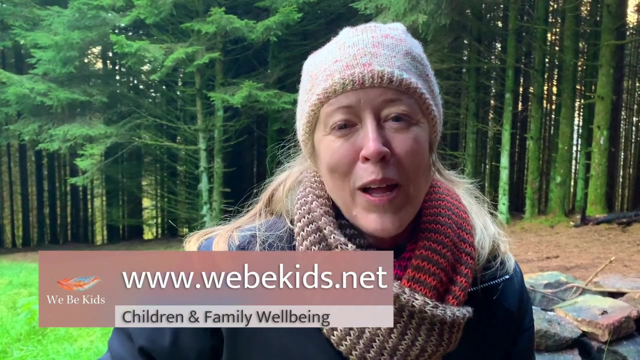 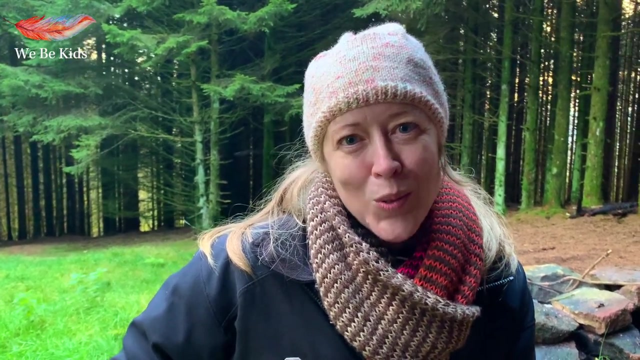 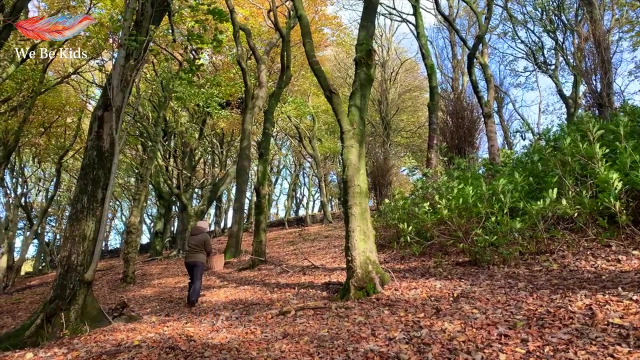 Hi, I'm Annie and I'm from Weeby Kids. Weeby Kids provides free nature resources online to help you and your family boost your well-being. Today, I'm going to be showing you how to make some beautiful autumnal leaf bowls. 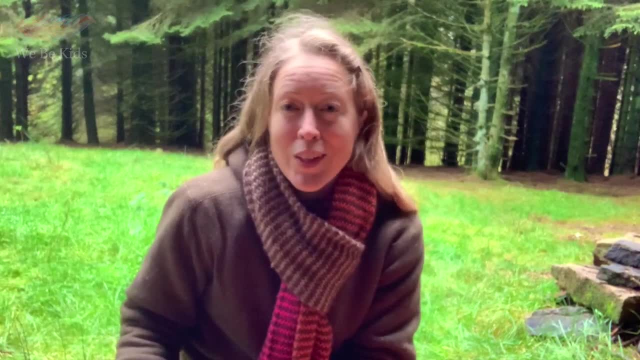 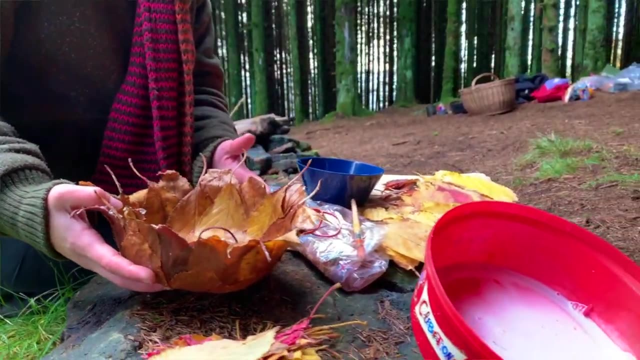 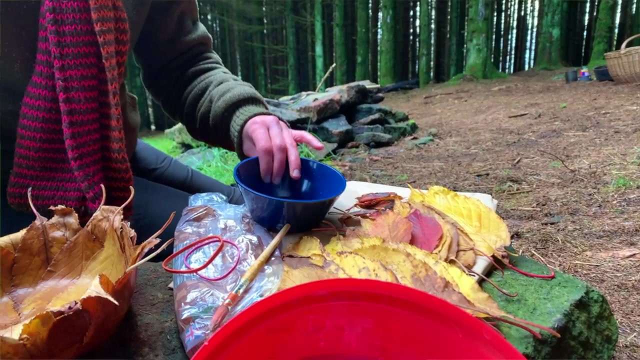 To make your own beautiful autumn leaf bowl, you need to make sure that you have some of the following resources: You need to have some PVA glue a brush. you need to make sure you have plenty of beautiful leaves that you can gather out on walks. 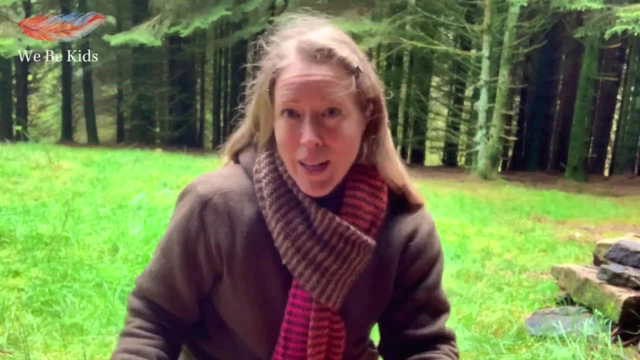 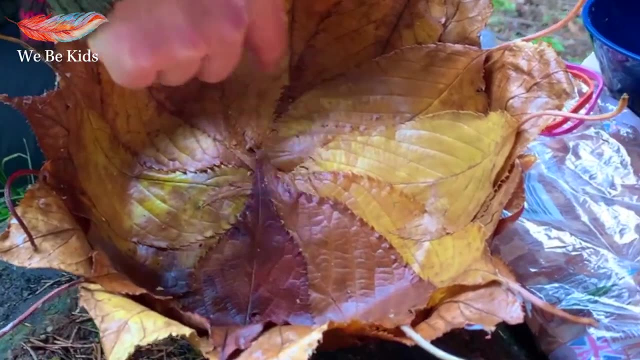 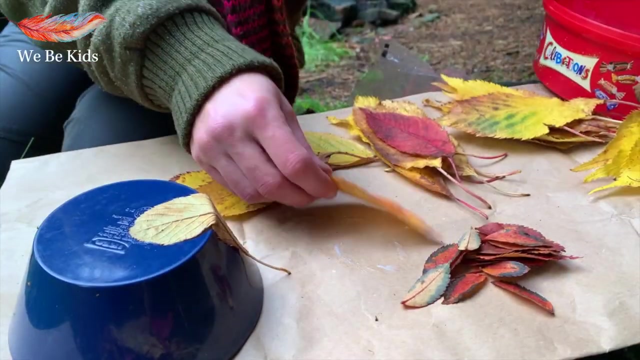 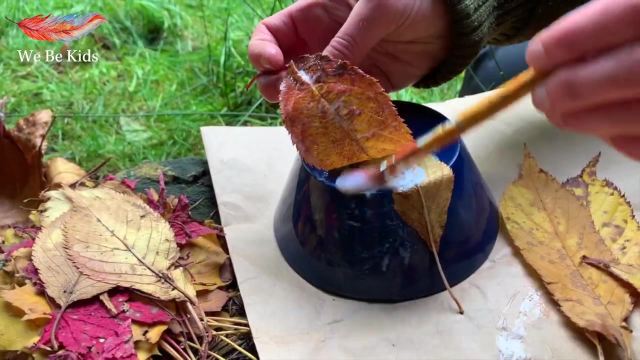 And you need to make sure that you have a bowl, preferably a plastic bowl or a metal one. To make your bowl, you need to consider both the layout of your leaves on the inside, as you are making, and also on the outside, When you're going to glue up your leaves. make sure that you apply glue nice and thickly. 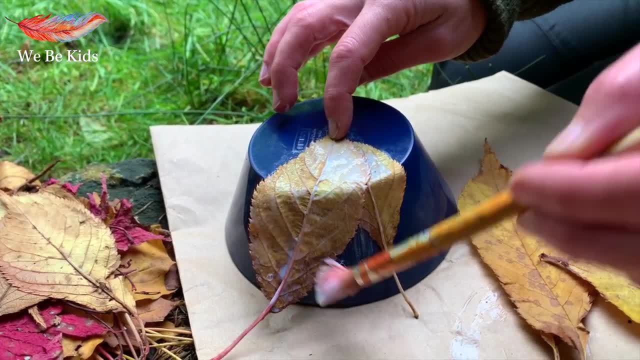 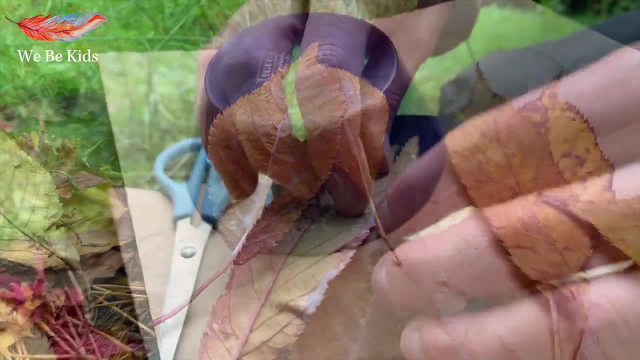 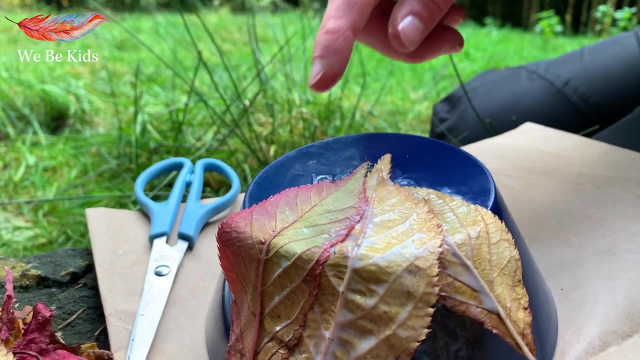 PVA glue tends to dry clear, so you don't have to worry at all about how it is going to look. In order to make sure that your leaves lie flat, you can end up with a little bit of a bump, which can be a bit of a problem. 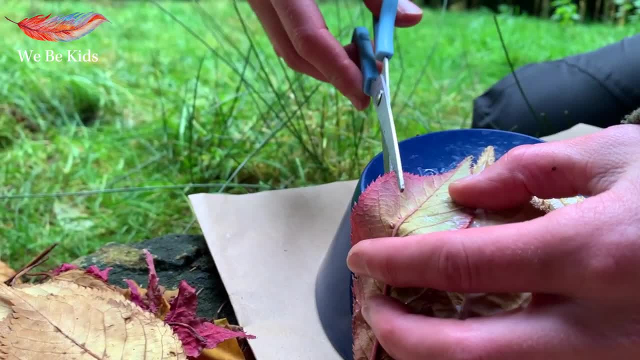 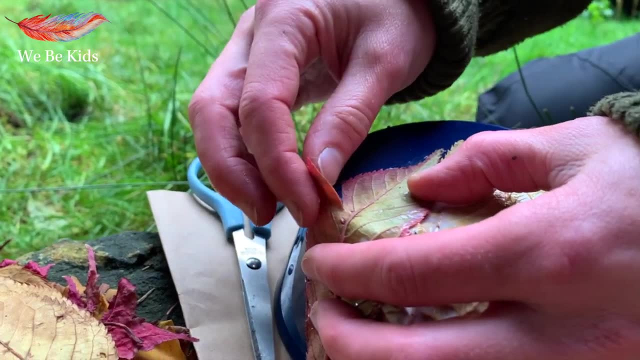 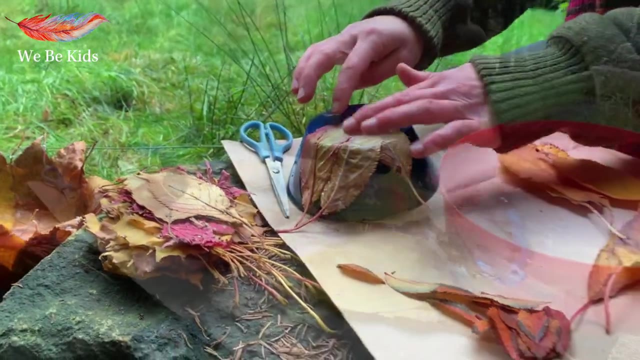 So if you take your scissors and snip a little bit in, lay the leaf down flat, fold it around on top of it, you get a much better fit to the shape of your bowl. But this will depend on the shape of your bowl. 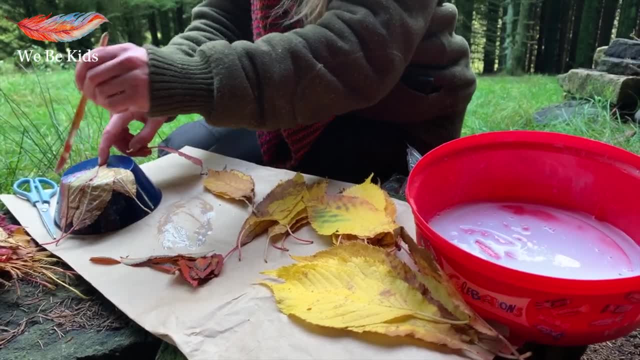 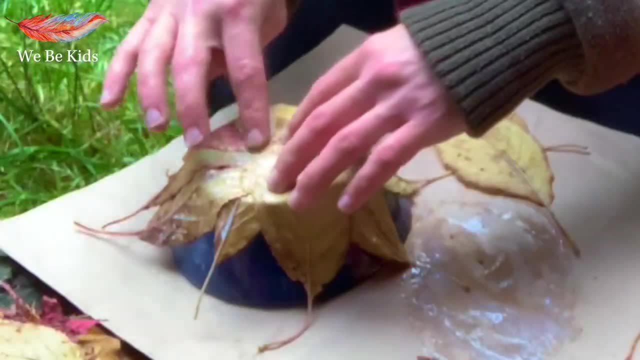 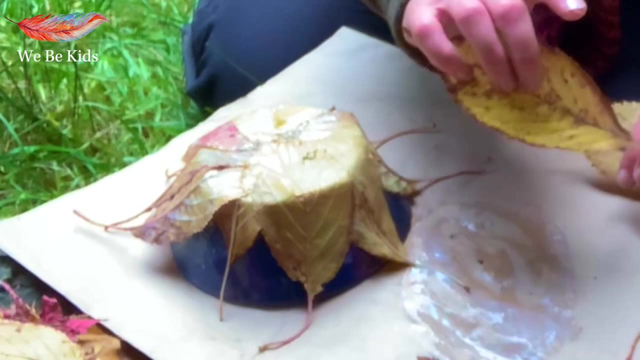 As you continue. note. it's really important to have the glue on this side as well as on the leaf you are about to apply. And now we've made our way around the whole bowl with one layer of leaves, which are actually with their outer facing upwards and that beautiful side facing down. 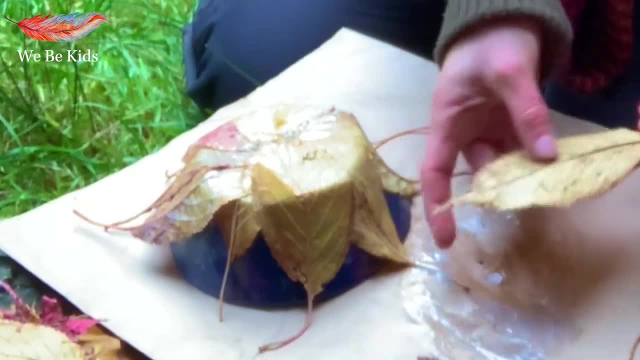 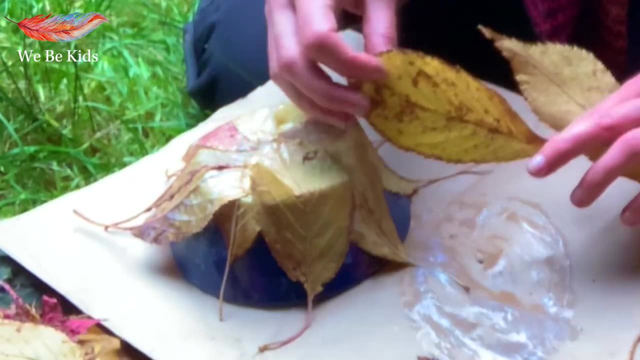 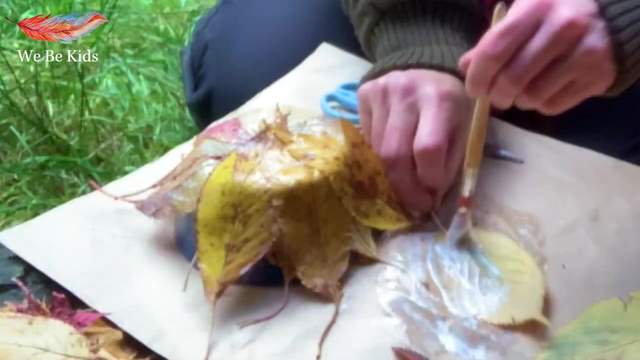 We're now going to turn that around and we're going to be placing now the inside on top of the inside and having the beautiful leaves on the outside. So this is going to make the outside of our bowl Consider the placing of these leaves. 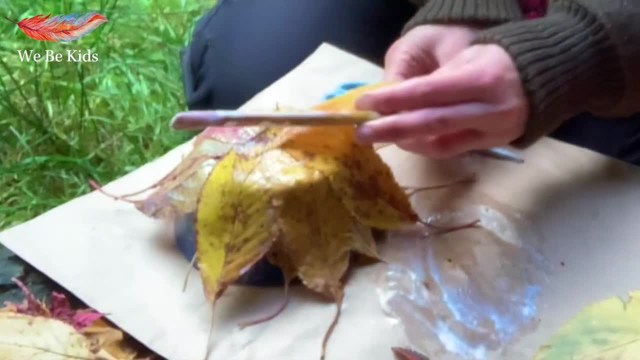 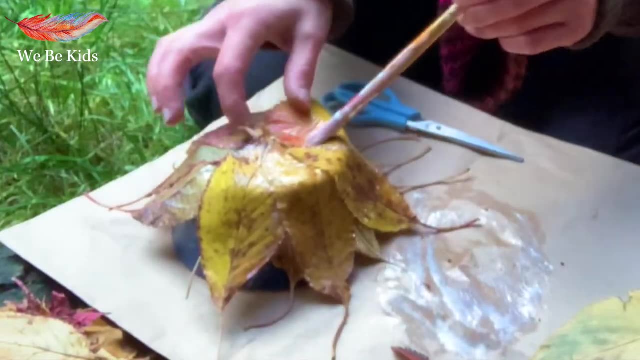 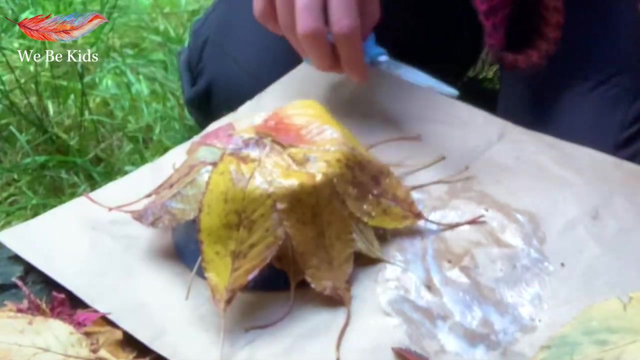 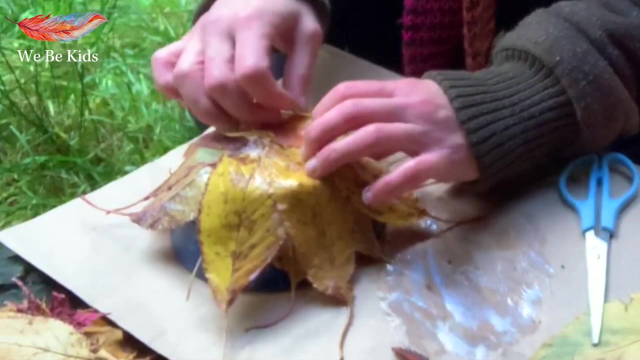 So perhaps they are going to sit in between the gaps of the first layer that you have already placed down And in the same way, you are going to need to consider making it fit. So if you need to use the scissor technique again, where you cut in and smooth it down, 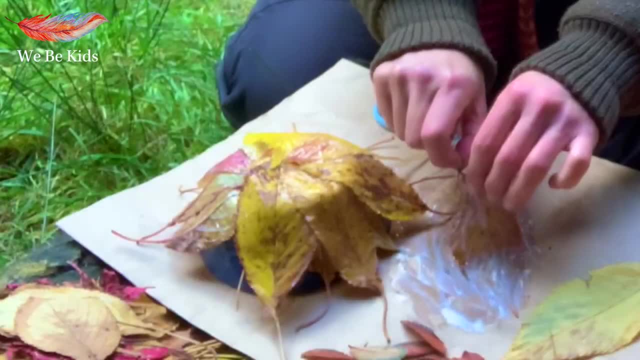 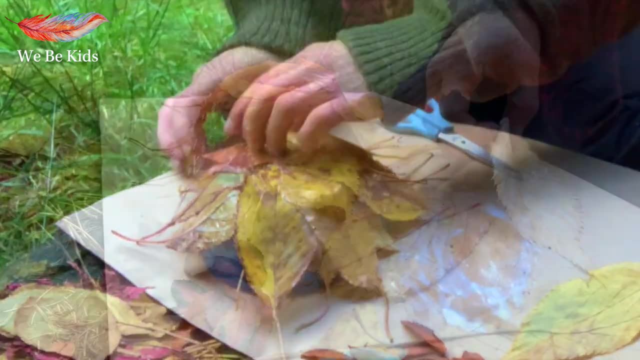 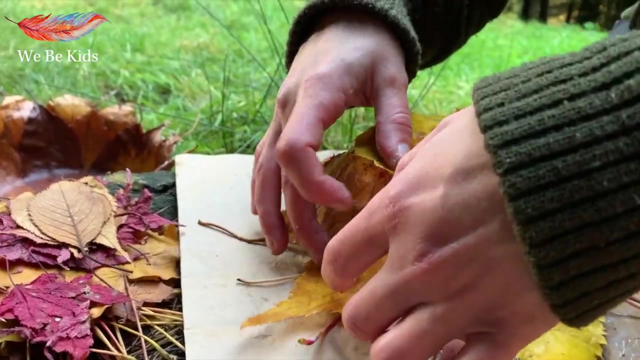 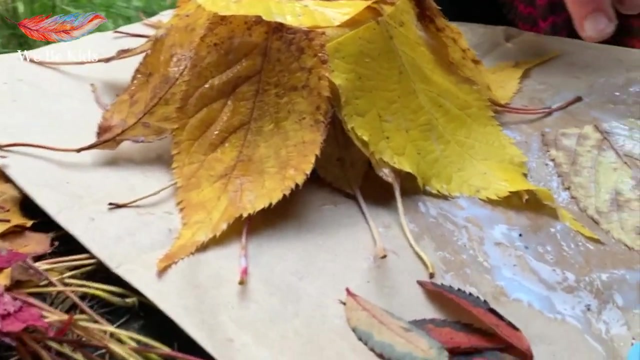 and round and on, then that's the way to go. Keep checking that they are all holding place. It's okay if they come loose a little at this stage and continue with gluing and sticking. Make sure that you are gluing down thoroughly as you go. 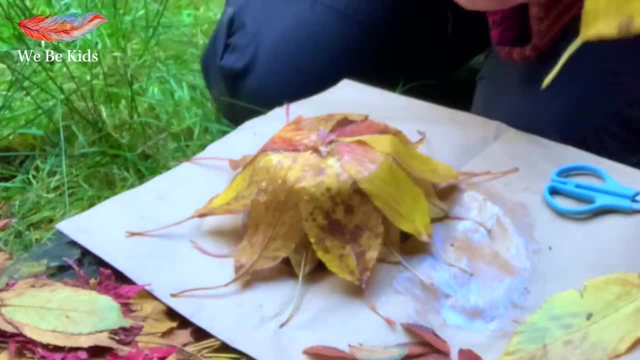 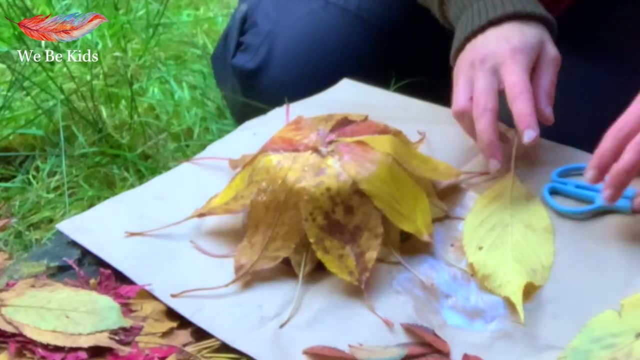 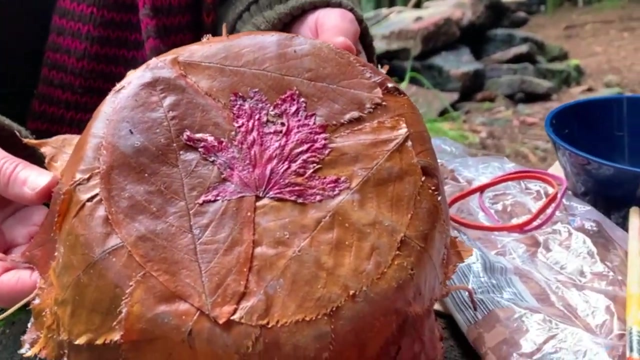 When we come to thinking about the base of our bowl and our final outer layer, it can also be useful to create shapes that fit the base. As you can see in our example, I've actually cut the bottom of the bowl And placed leaves on, and then cut any excess off the edges. 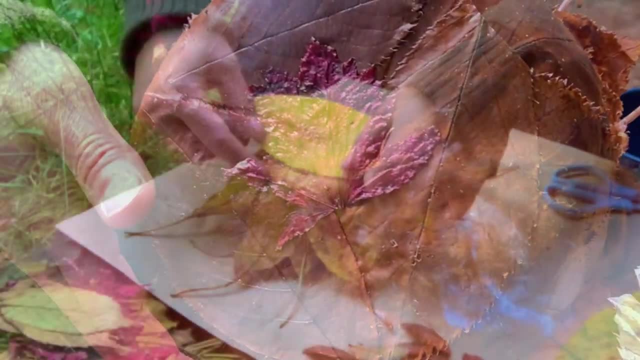 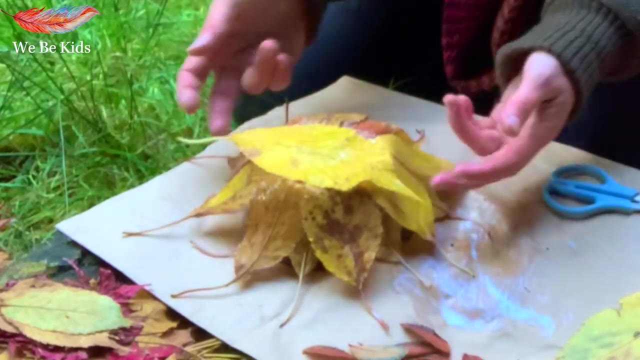 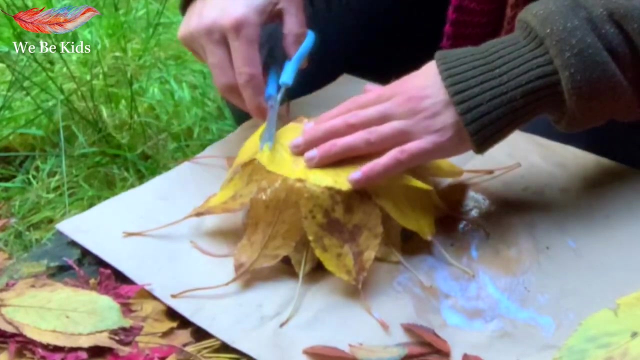 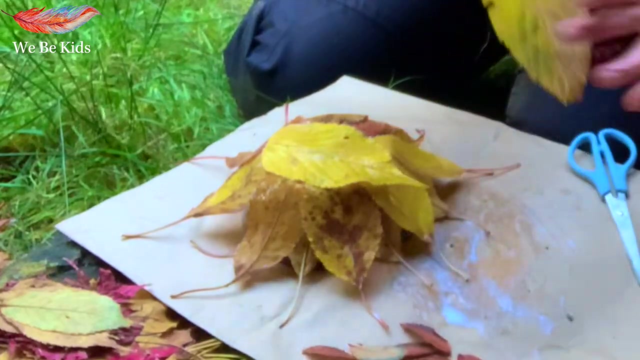 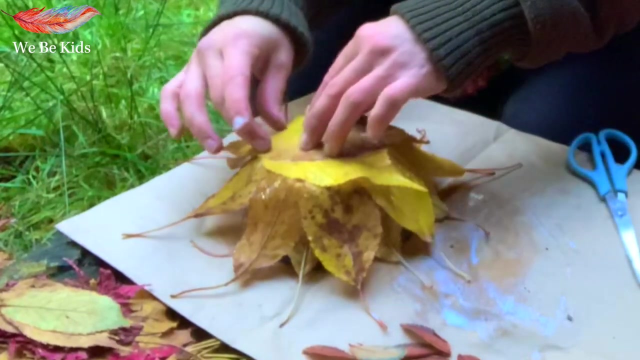 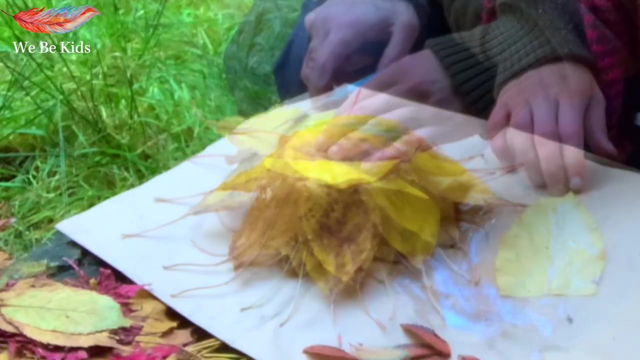 So I can place my leaf on the end there and, as you can see, the ends there are sticking up over the edges and I can just trim with my scissors to fit the shape. I'm going to lay that down on top. What this helps us do is also seal all of those little pieces that we've had to cut.